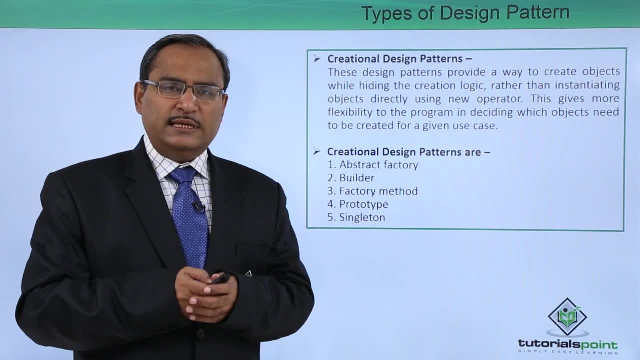 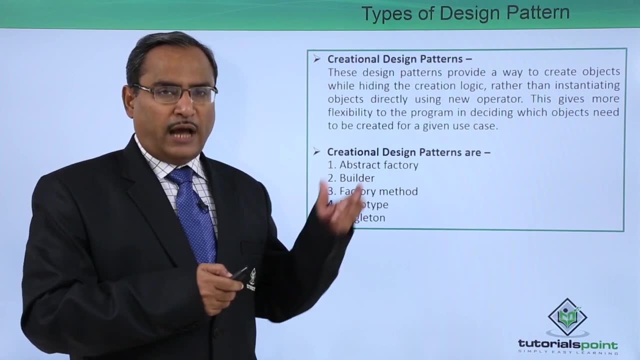 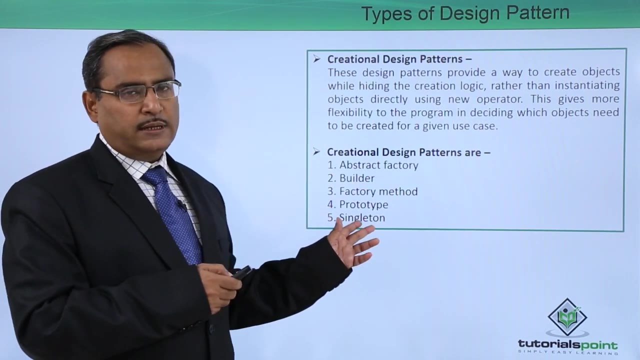 for a given use case. So what is the use case? Use case is nothing but one functional requirement of the software. So which object is to be created for a given use case? we can decide on that. So creational design patterns are having. following design patterns are coming. 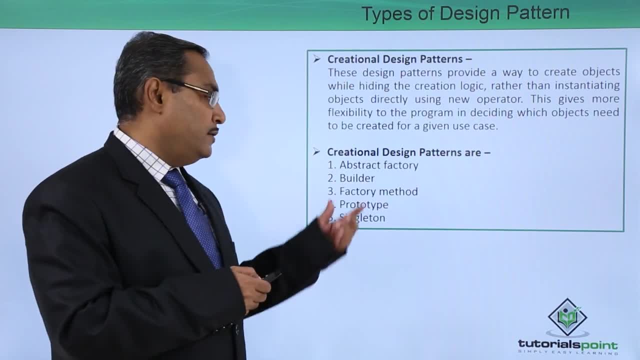 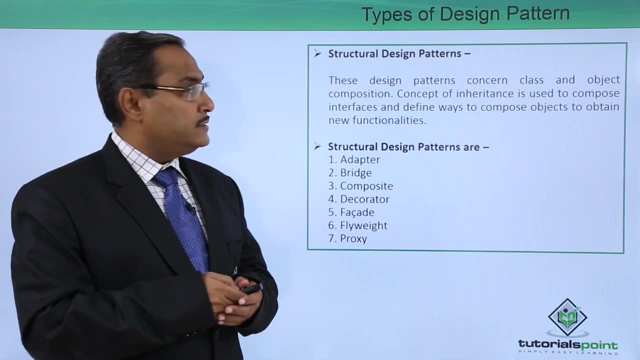 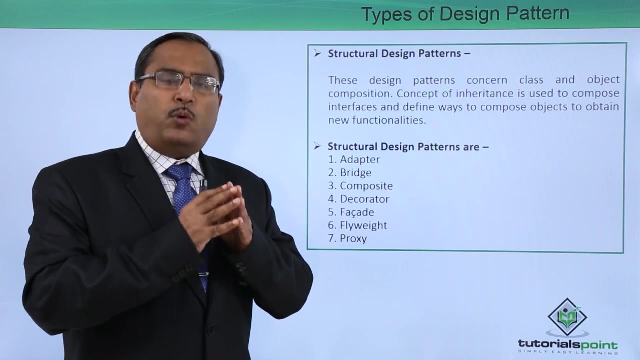 under this category. So abstract, factory builder, factory method, critical design, prototype and single turn design pattern. So now let us go for structural design patterns. These design patterns concern class and object composition. So that means object of one class will be used in another class, So that 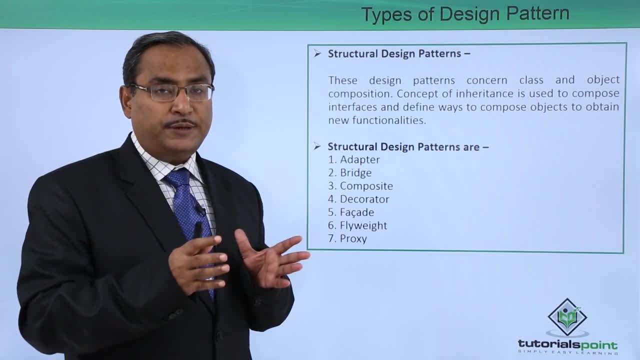 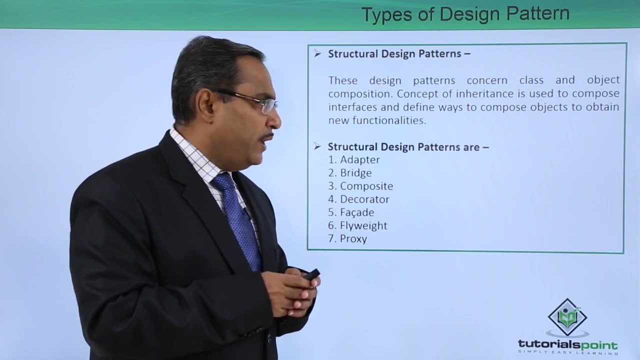 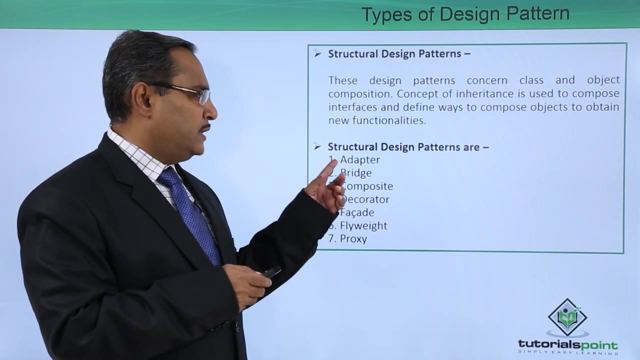 is known as the object composition. that is a hazard relationship between two classes. So concept of inheritance is used to compose interfaces and define ways to compose objects to obtain new and new functionalities. So under this structural design pattern we are going to have this set of design patterns. 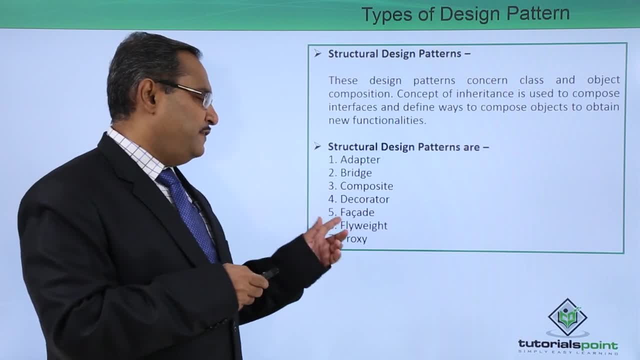 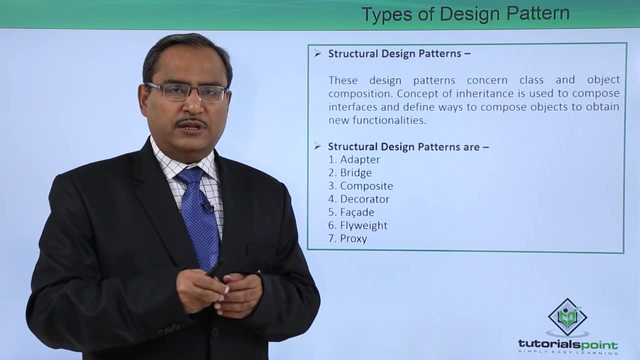 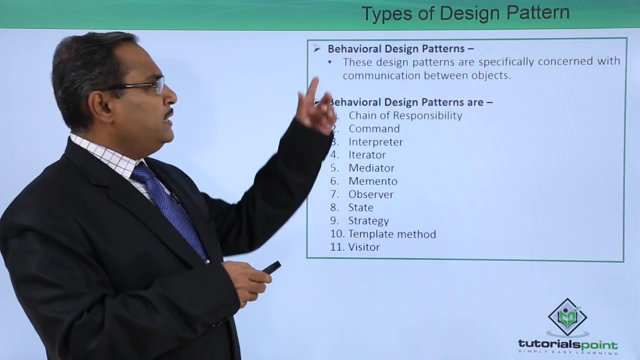 so that are: adapter, bridge, composite, decorator, facet, flyweight and proxy design patterns. We will be discussing each and every one in our tutorial, with the detailing, with the detail concept and with the implementation in our Java code. Next one is the behavioral design patterns. These design patterns are especially concerned. 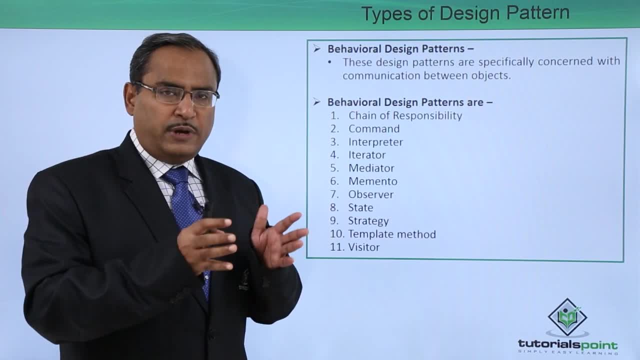 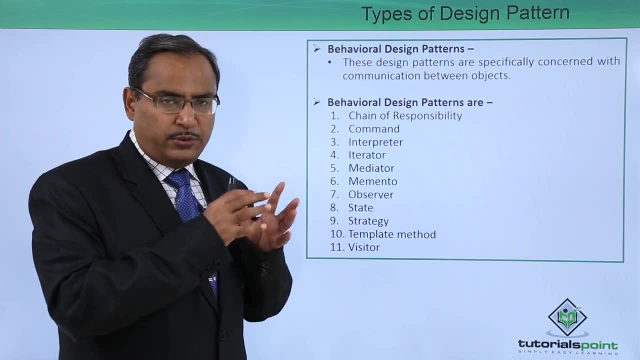 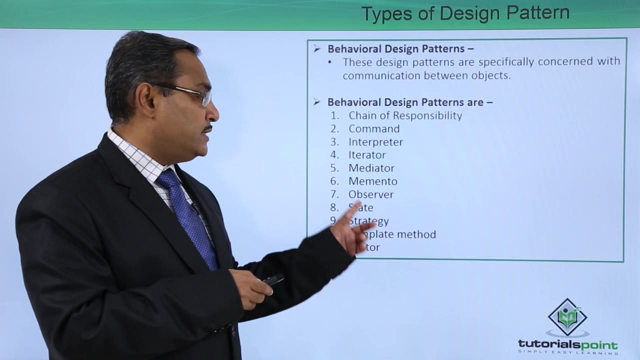 with the communication Whenever you require communication between objects. whenever you require communication between objects, then you shall go for this specific category. Under this behavioral design pattern category, we are having the following design patterns. So they are chain of responsibility: command, interpreter, iterator, mediator, memento, observer. 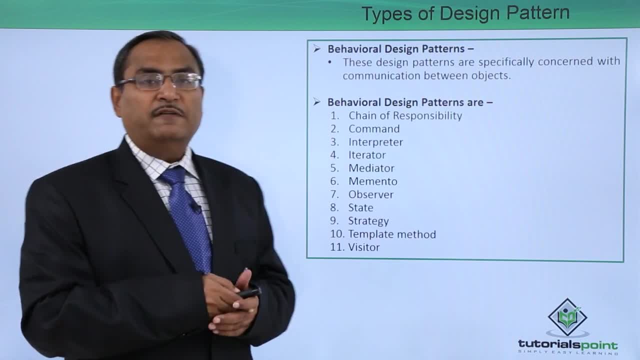 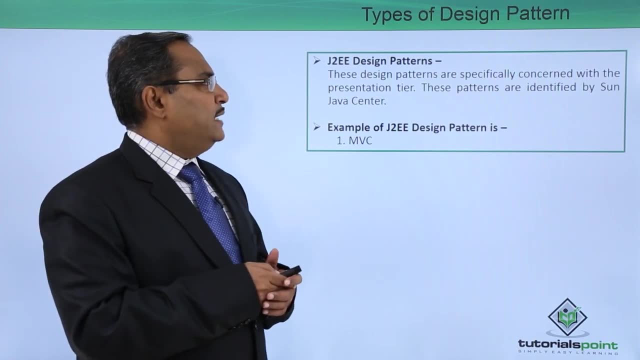 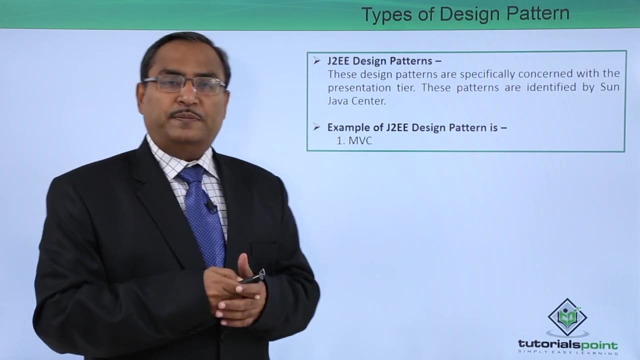 state strategy and template method and visitor design patterns. We shall be discussing each and every one in our tutorial. So in case of G2E design patterns, These design patterns are specifically concerned with the presentation tier. So what is the presentation tier? 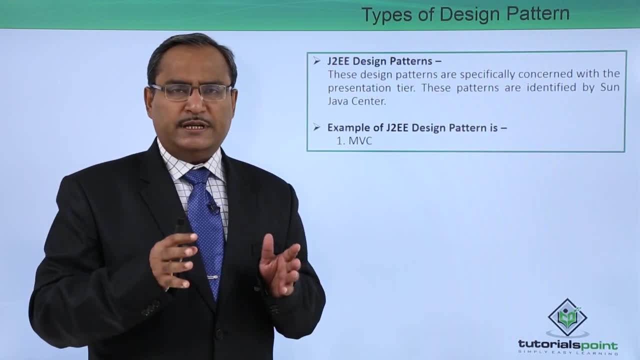 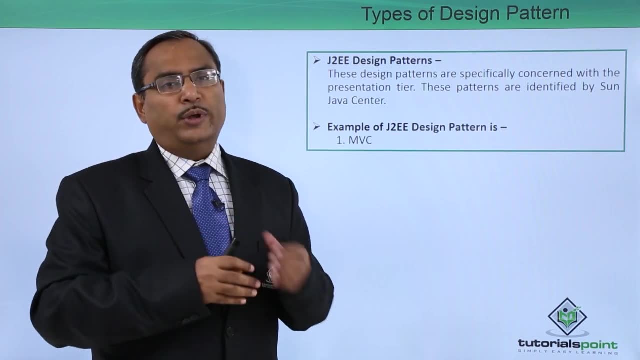 We know that we are having in our software. we are having mainly three different tiers. One is the data tier, next one is the logic tier and the last one is the presentation tier, which will be interacting with the user through some user interface. 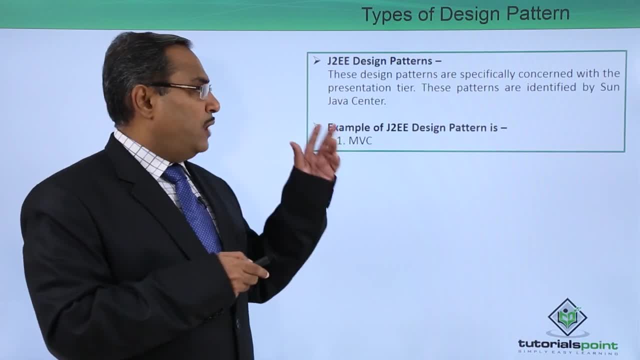 These patterns are identified by SAN Java center. So under this G2E design pattern in our tutorial we shall cover the MVC pattern. So let us start with the G2E design pattern. So this is the G2E design pattern.